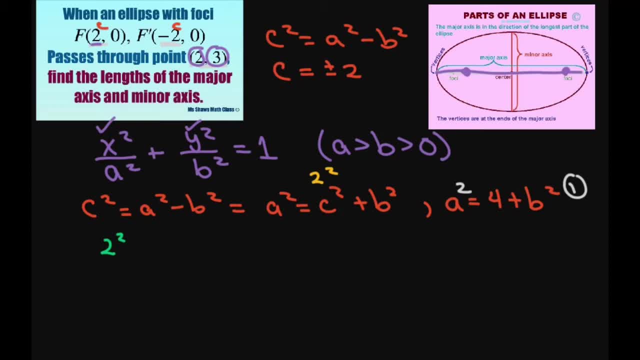 So I'm going to get 2 squared divided by a squared, plus 3 squared divided by b squared equals 1.. Now my common denominator is going to be a squared times b squared. So if I just multiply through everything by a squared times b squared, 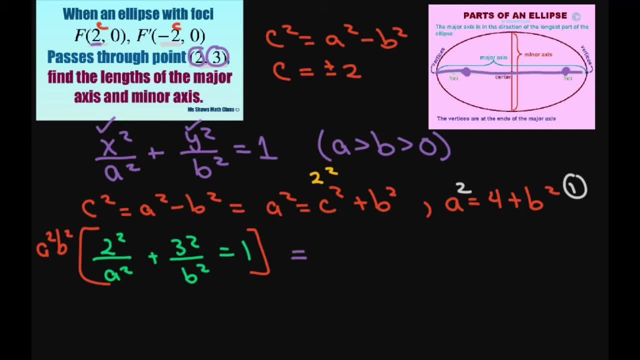 I'm going to get This equals. this will cancel out. You'll have 4b squared And then for this one, the b squared will cancel out and give you 9 times a squared. And then you have to multiply these two and you get this: equals a squared times b squared. 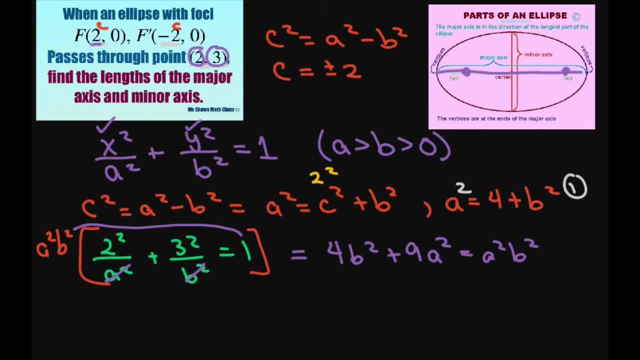 Alright, and if you want, you can switch these around, But let's go ahead and substitute in our a squared Into this. So this is equation 2, and we're going to substitute 1 into 2.. Therefore, I'm going to switch these around. 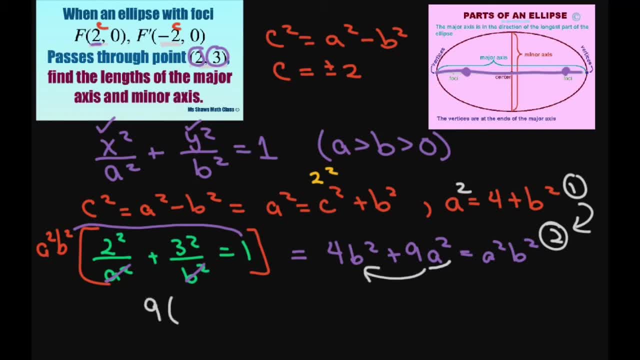 So we're going to have 9 times a squared, So a squared is 4 plus b squared, And then we still have our plus 4b squared And then we have a again. So a is 4 plus b squared. times b squared. 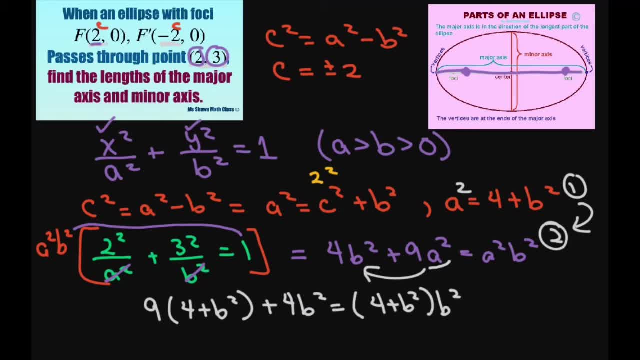 Now, simplifying all this, we're going to get b to the power of 4 minus 9b. squared minus 36 equals 0. So, basically, I just took care of this side and this side and moved everything over to the left-hand side. 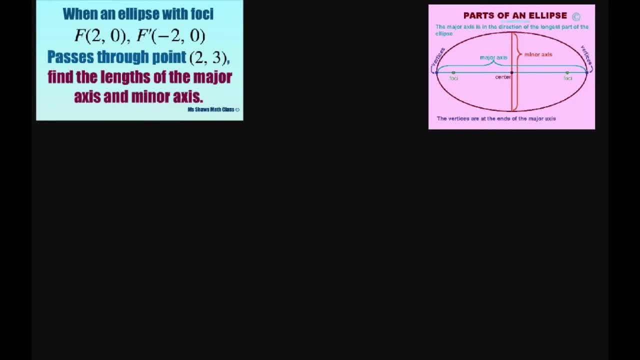 Okay, so we have b to the power of 4 minus 9b squared, And then we're going to have b to the power of 4 minus 9b squared minus 36 equals 0.. Factoring this, this gives us b squared minus 12 times b squared plus 3 equals 0.. 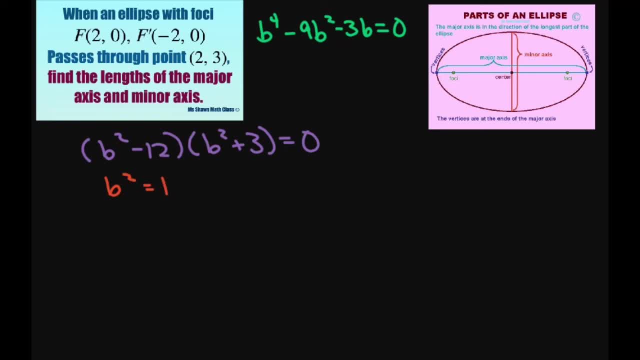 Therefore, we have b squared equals 12 or b squared equals negative 3. Now our b squared has to be positive, And so that knocks that out, And that's because our b has to be positive. That's how we set it up.